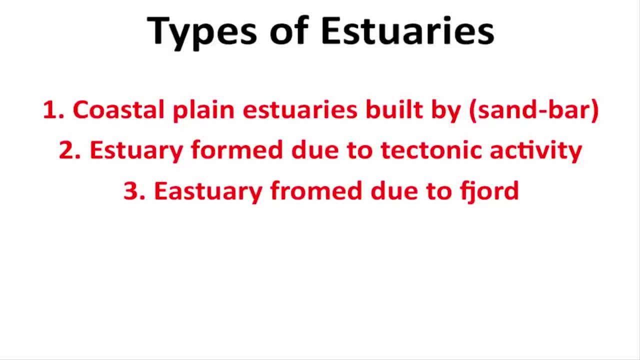 The answer to this question depends on the types of estuaries. There are three different kinds of estuaries, each created in a different way. I am going to explain each of them one by one. The first one is Coastal Plain Estuaries built by Sandbar. 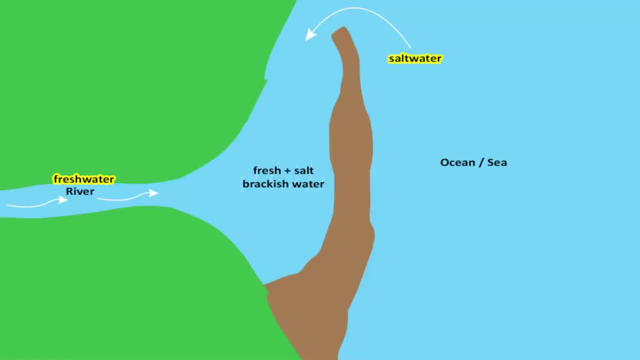 If you ever go to a coastal area, you will find a small pool of water that gets separated from the ocean. This is called an estuary. It can also be called a lagoon. What you have to understand is that when a river joins the sea or ocean, obviously. 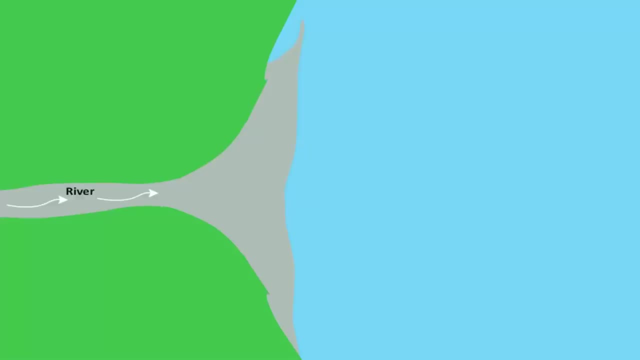 the land elevation towards the sea has to be low. That is how there will be a gentle slope which will allow the river to meet the sea. We also know that the ocean water continuously hits the coastline Along the way. it brings, as well as washes away, a lot of sediment. 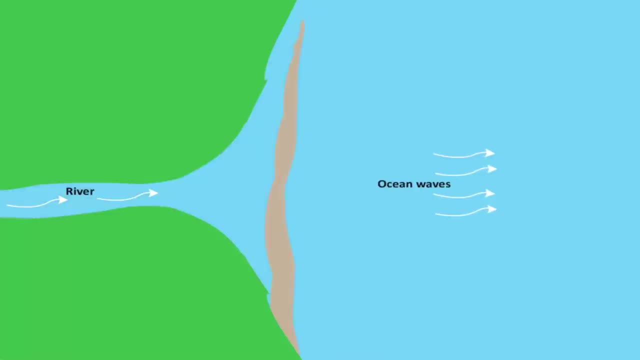 Now, due to continuous hitting of waves, the sediment churns and turns into a sand ridge or a sandbar. As a result, a small pool of water gets separated from the ocean. This is called a lagoon. This is also how a coastal lagoon is formed. 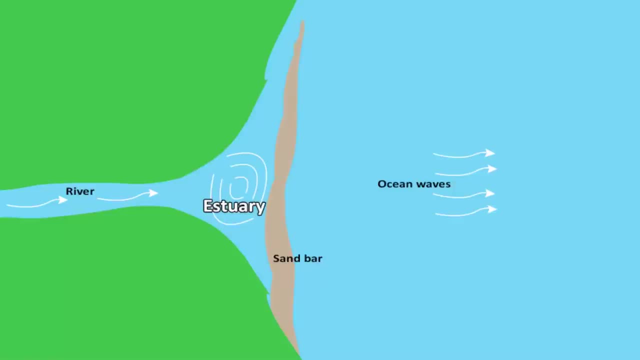 But in this video we will call it a coastal plain estuary. This estuary is connected both to a fresh water river and also to a small stream from the ocean for getting its salt water supply. That is how this estuary will get its brackish water supply. 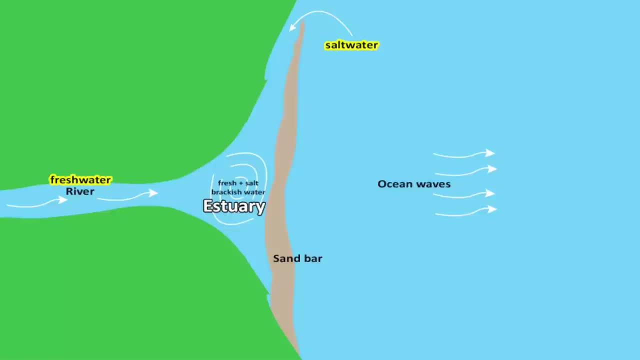 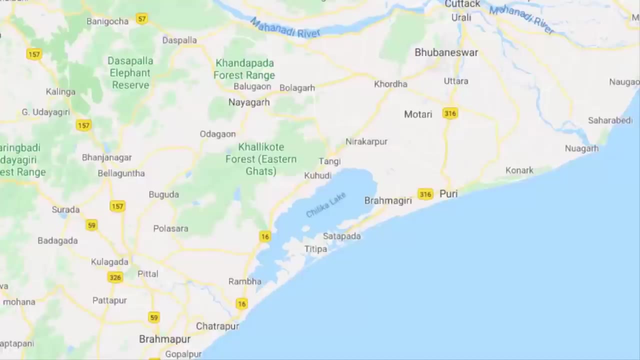 Apart from this, there is another way this coastal estuary get its water, and that happens when the sea level rise. The most famous lagoons in India, like the Chilika Lake, the Kaliweli Lake, the Kerala backwater, 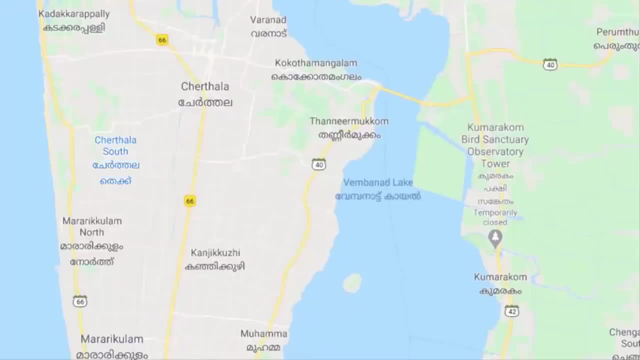 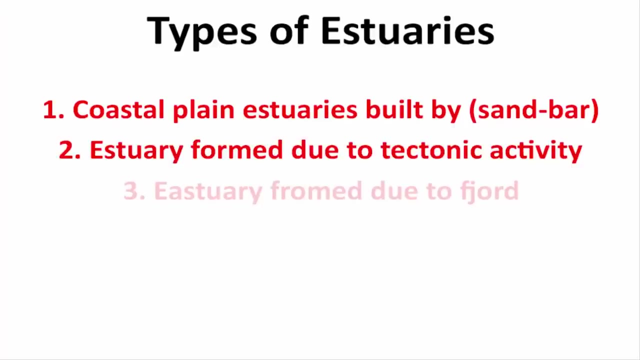 Pulikat Lake and Vembanad Lake. These lagoons can also be called as coastal estuaries. The second kind of estuary is formed due to tectonic activity. When two tectonic plates collides with each other, slides against each other or moves. 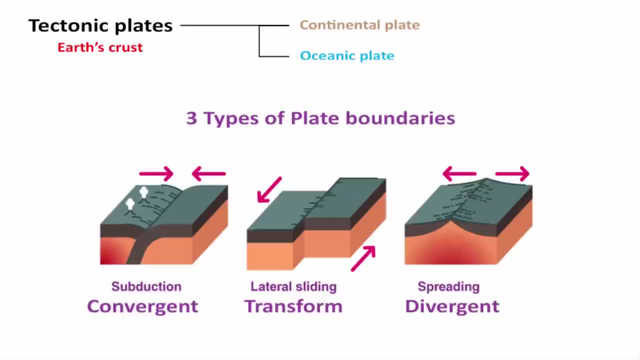 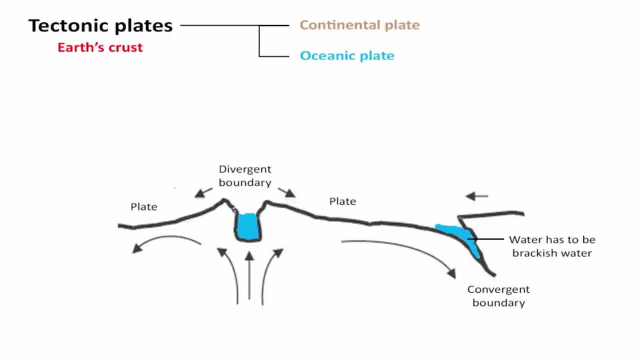 apart from each other. that is also how estuaries are formed, Because in all these three situations you will find a land depression. When this land depression gets filled up with water, that is also an estuary. A good example is the San Francisco estuary. 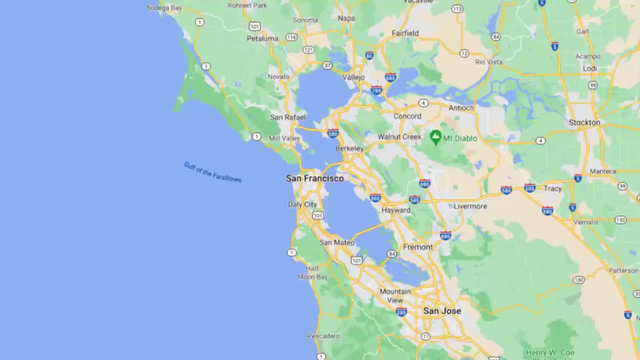 Here the water is a mixture of seawater and freshwater. Plus, this estuary is a partially enclosed coastal body of brackish water. Now you may have a question. well, it is called a bay, so does it mean even Bay of Bengal is an estuary? 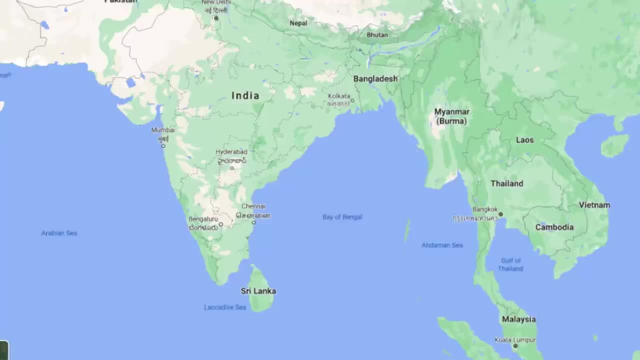 There are a lot of rivers that flow into the Bay of Bengal. Plus, the water of Bay of Bengal is also part of the Indian Ocean. That means a mixture of saltwater and freshwater is there, So is it right to call Bay of Bengal an estuary? 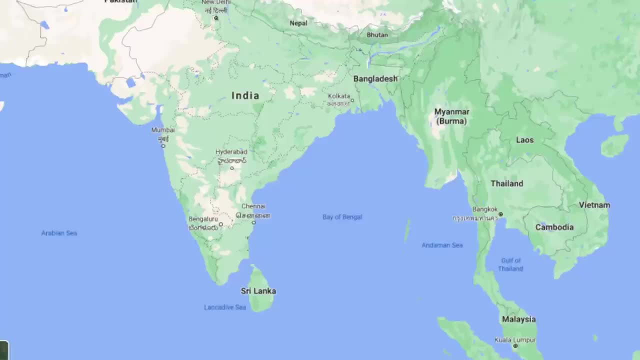 The answer is no. I mean, just think about it. In what category of estuary will you put Bay of Bengal? Bay of Bengal was not formed due to any tectonic activity. It is not even enclosed. There is no sandbar. 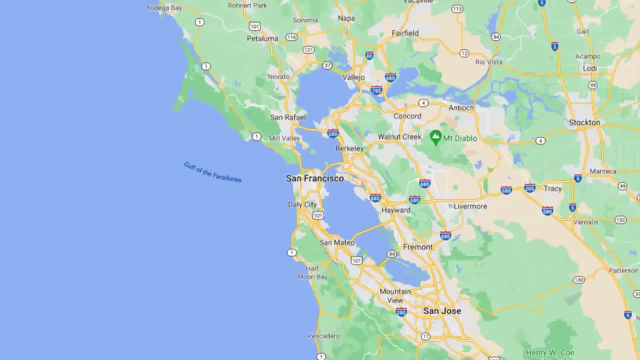 But if you look at the San Francisco Bay, first of all, if you see it is a partially enclosed coastal body of brackish water. That means there is so much of landmass that encloses this bay. There is only this little opening called Golden Gate, from where the Pacific Ocean saltwater 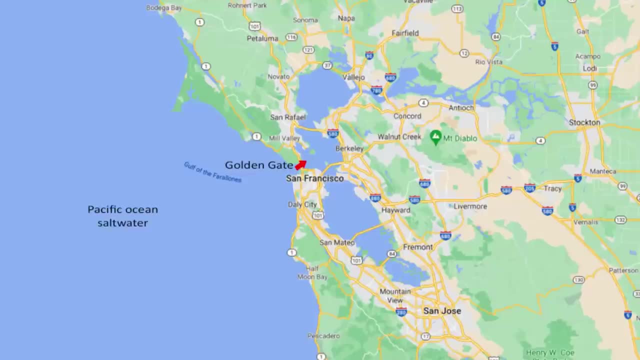 is coming in On top of it. San Francisco Bay is located on the San Andreas Falls. The San Andreas Fault is the sliding boundary between the Pacific Ocean Plate and the Northern American Plate. Because of this kind of tectonic activity, this entire San Francisco Bay has been formed. 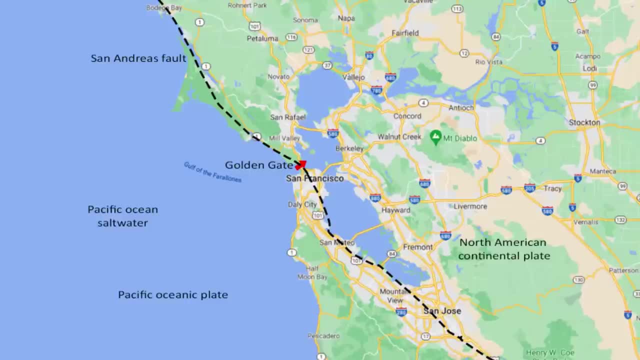 which has eventually got filled up with both fresh water from rivers and salt water from the Pacific Ocean. So the most important thing that you have to remember about an estuary is that it needs to have brackish water, And the third type of estuary is formed due to fjord. 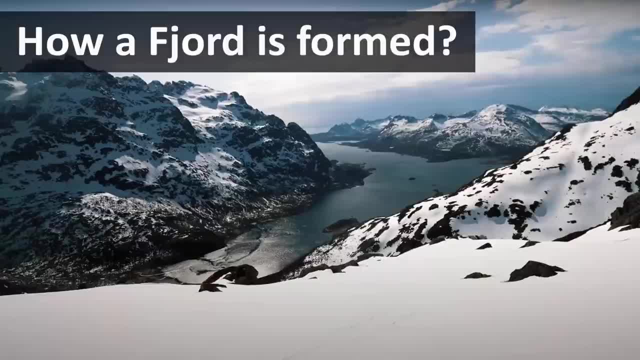 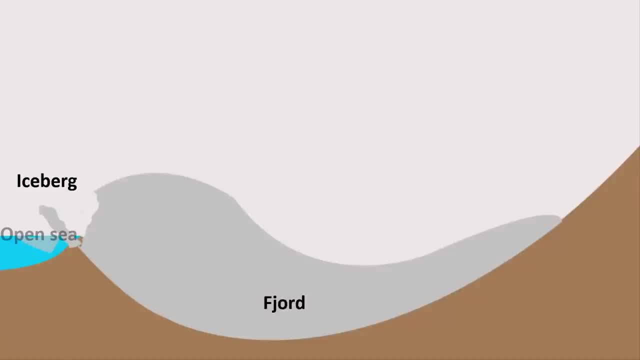 I already have a video in which I have explained how fjords are formed. Glaciers move downslope very slowly over time and it carves a valley and forms a land depression. This land depression gets filled up with sea water. So this is how a fjord is formed. 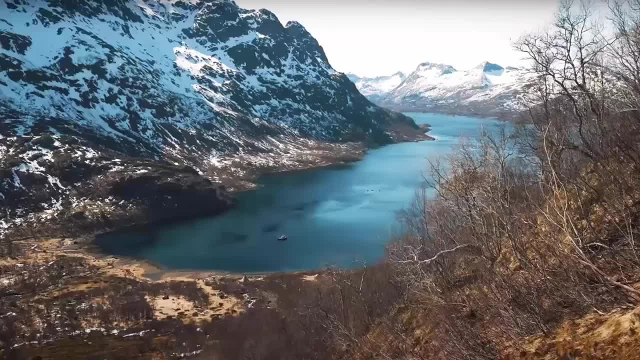 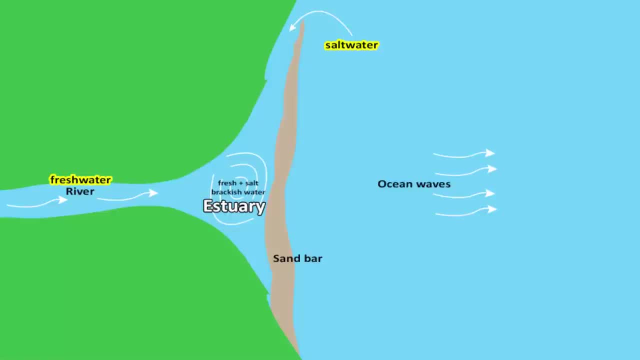 Now, if this fjord gets fresh water from nearby glaciers and mountains, only then we can call it a fjord estuary In the end. all you have to remember is that an estuary should have brackish water. There has to be a land depression. 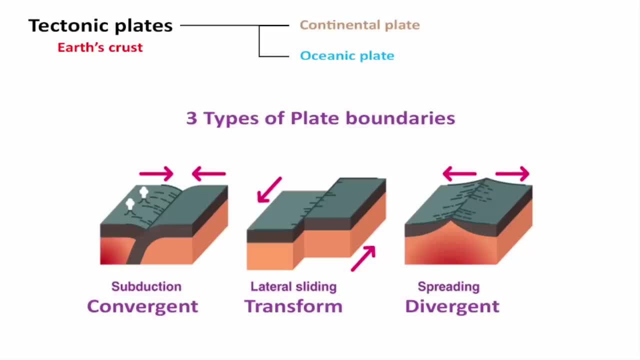 Or some kind of natural water Or some kind of natural blockage that is caused due to tectonic activity, glaciers or ocean tides that create sandbars.